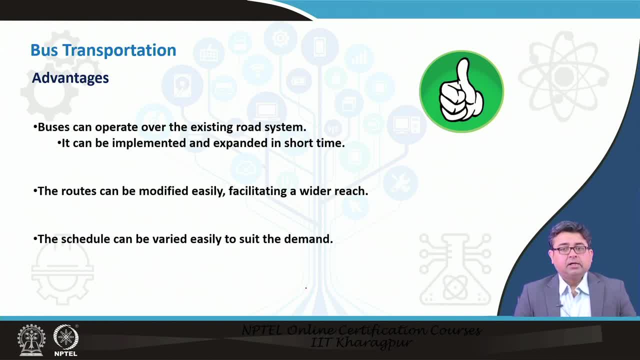 bus transportation has Now. there are other advantages as well. The routes can be easily modified. It could be rerouted based on newer developments that are coming up. So, for example, you have an existing bus route line or a bus route but a new residential development comes up. You can easily extend that line to that new residential. 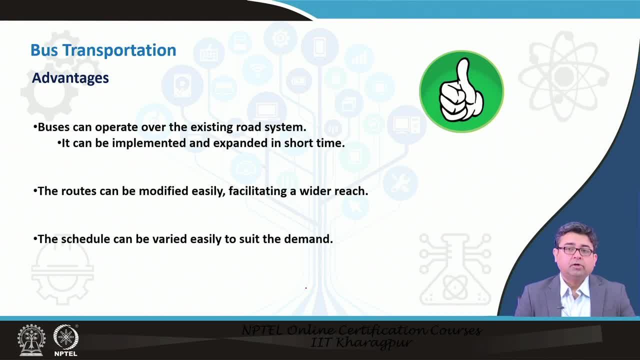 area. You do not need a whole lot of infrastructure to put in to in order to extend it. So the the next advantage is the schedules can be varied, So you can have multiple schedules. you can during the day, during the month, during the. 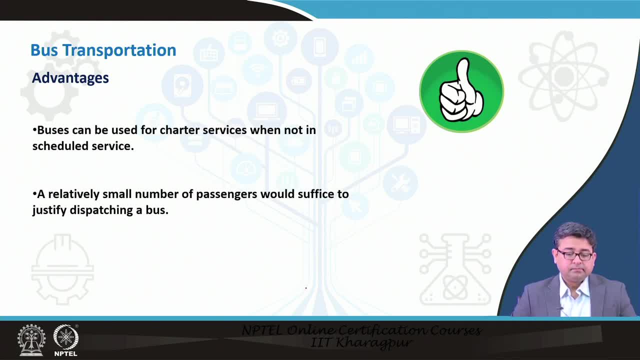 year, you can have varied, varied schedules as well. Then the other advantages: when the fleet, the entire fleet, is not required to run on on a bus route or on a bus network, you can charter those buses, So you can utilize your fleet in different manners. 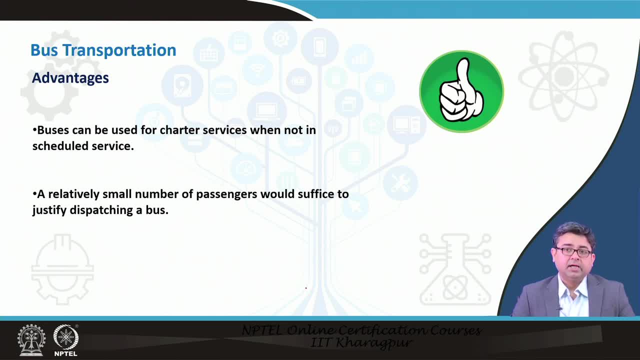 So you, so that they are not laying unutilized and they are not generating any revenue. So they can be used for charter services and and relatively less demand. relatively a lower amount of demand usually suffices for dispatching a new bus service. 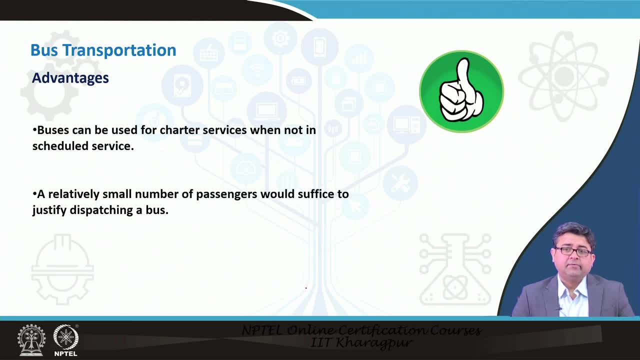 For example, only a 20 to 25 number of Passengers is sufficient per hour in order to justify a new bus. So, whereas the other larger public transportation systems require a higher demand, or a greater demand just in order to justify a new system, 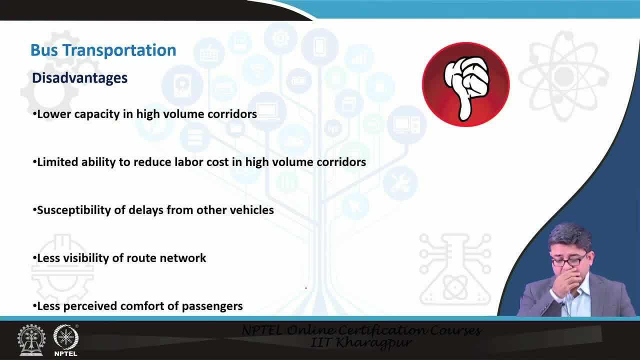 So bus transportation has these advantages. At the same time, it has several disadvantages as well. One is because they run on existing routes or existing roads, they are susceptible to delays. So they are susceptible to delays not for their inherent reasons, but for reasons of 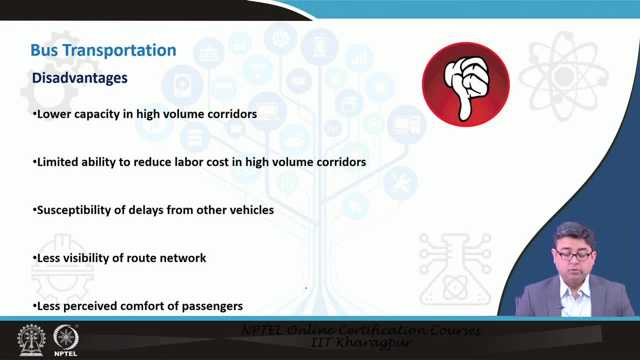 other modes of transportation that are running on the roads. Then it is also a less visible route network because it runs on existing infrastructure or on existing roads. it gets hidden among see all the other traffic and you. usually it is not very conspicuous. So you will see many cities paved roads. 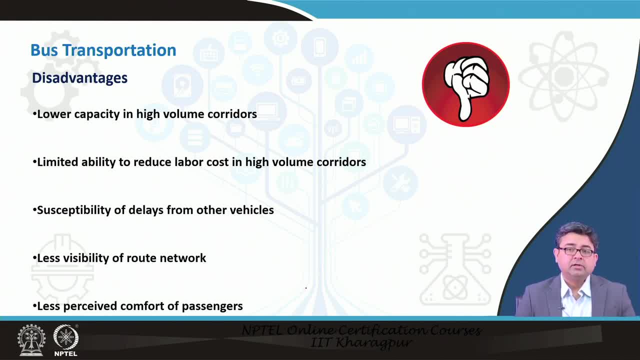 So you will see many cities paved roads. So you will see many cities paved roads. They will be painting their buses a certain color So as to make them stand out in in the traffic. otherwise they kind of blend in and they 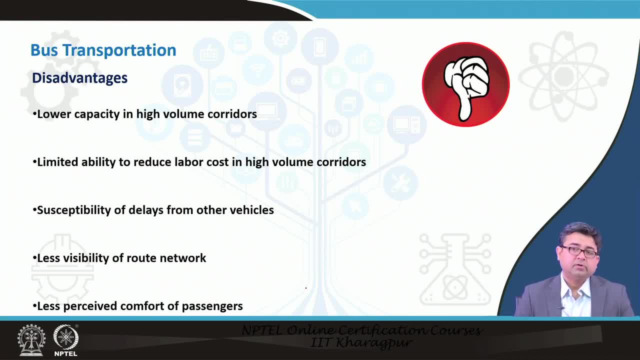 you cannot easily spot the bus that you want to get on. The other big disadvantage, which is more to do with the perception of the people, is that people feel that bus transportation is less comfortable, So they always have this feeling on their in their mind that it will be crowded. 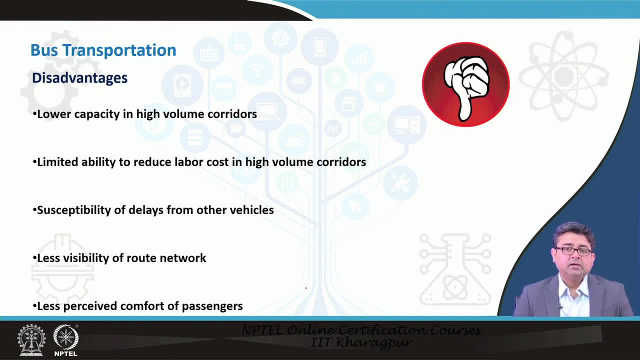 They will not be able to go and they want to walk. They will not be able to go and walk. You would not find a seat. the infrastructure may not be of highest quality, So this perception is something that is associated with bus transportation. 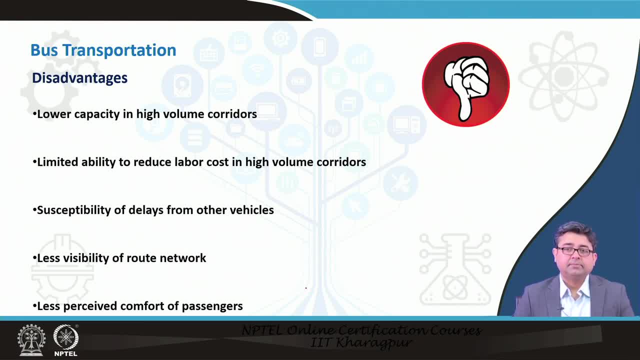 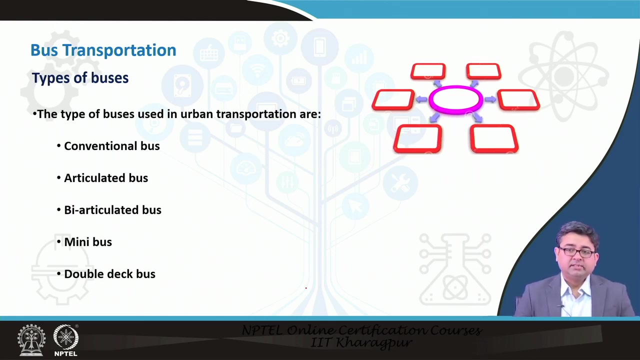 And also for standard buses. sometimes what happens is, if you do not have high capacity buses, then they do tend to get overcrowded and the capacity usually cannot be easily added on because you need. the fleet size is almost many times constant. So those were the advantages and some disadvantages of bus transportation. 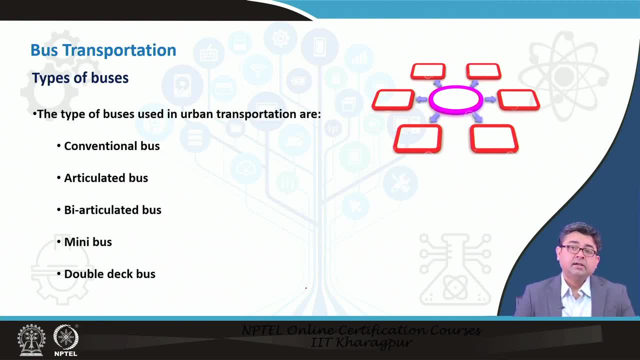 Now you need to know what are the different types of buses, because for a particular route or for a particular network, you need to run only those type of buses that will cater to the demand on that route. So you do not need to. 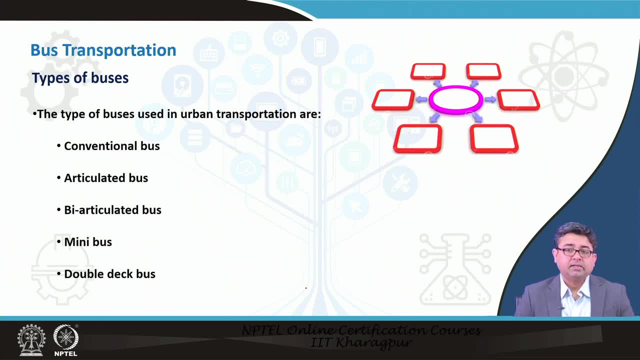 So you do not need to run high volume, high capacity buses on routes that have very few people who use them Similarly or alternately. you do not. you should not have a low capacity buses, such as mini buses, on routes that have high demand. 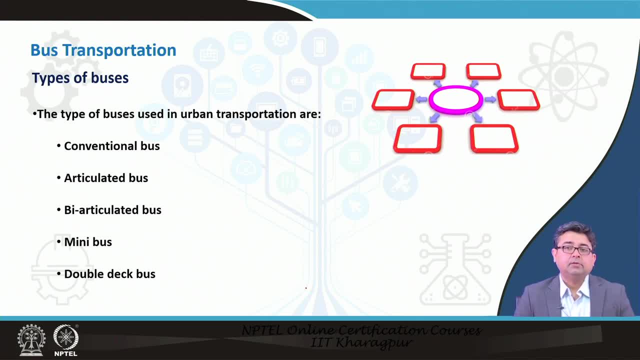 So once you are aware of what are the different types of buses, this will help you plan accordingly. Usually, you will see there are conventional buses, 40 foot buses. then there are what are called articulated buses. These are bi-articulated buses, mini buses and double decker buses, which are now limited. 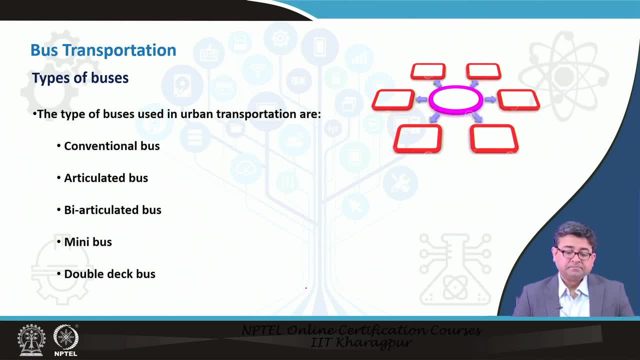 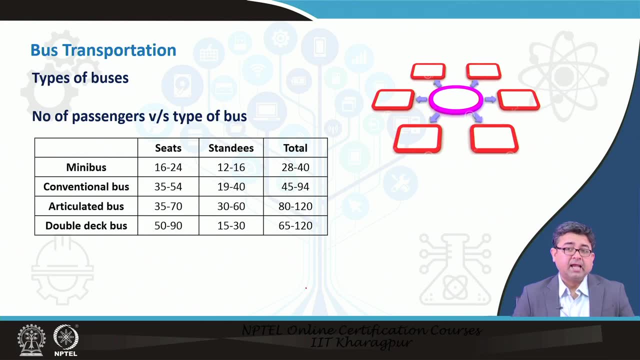 in some number of cities in India and also across the world. This is: this gives you a kind of an example of how many passengers can travel sitting and standing in each of these buses. So you would see, a conventional bus has anywhere between 35 to 54 seats it can accommodate. 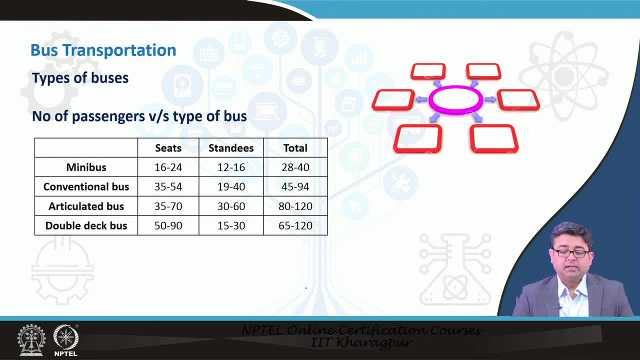 or it should accommodate 19 to 40 people. So a total of 45 to 94 people can be accommodated in a standard bus. So this is the general practice that should be followed. Now, it is not to say that any of the buses in India carry more than this or less than. 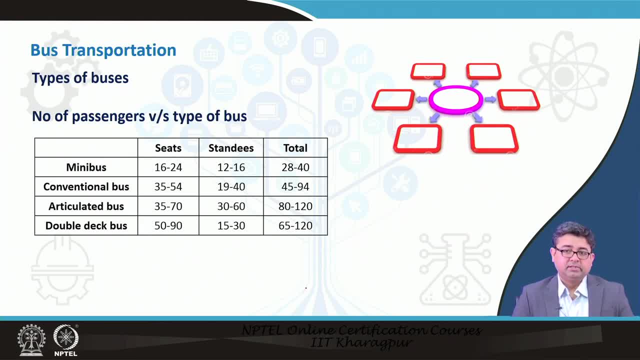 this, but this is what we generally recommend, or we is generally noted, when it comes to different capacities for different buses. This takes into account The revenues that are generated. this takes into account the comfort of the people that are riding those buses and some other factors. so this is a general guideline. 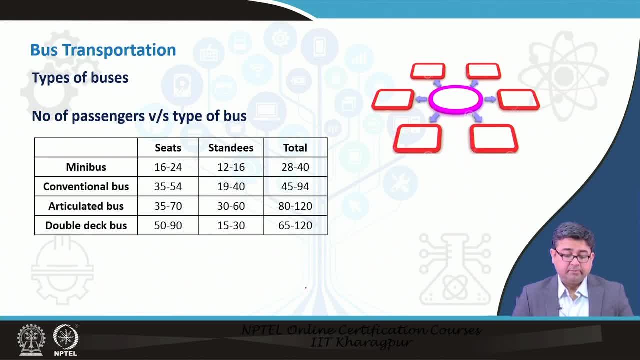 Now you see, articulated buses can take many more people. similarly, double decker buses can take- accommodate many more people, but they have their own issues. such as articulated buses require a very large turning radius, so they may not be able to get into the narrowing. 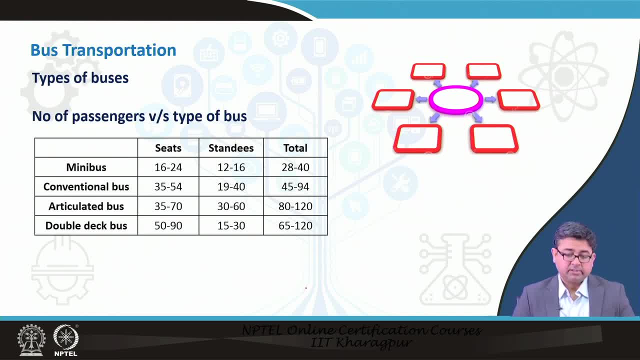 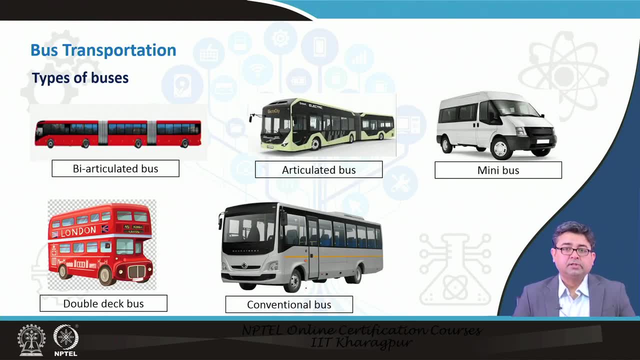 the narrow streets, urban streets in your residential areas, so on and so forth. Here are some pictures of different type of buses that I was discussing: A conventional bus, double decker buses, articulated and by. articulated buses are something new that are coming up in some of the cities which are heavily investing in improving that bus. 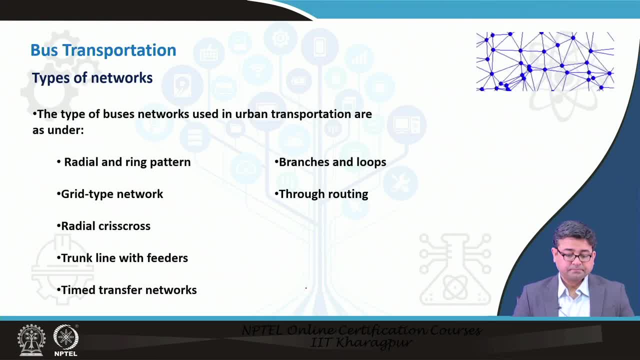 transportation systems. Well, first of all, an actual bus so, for example, you can transport around transportos accordingly to different areas. orthodoxy, particularly with feel free. 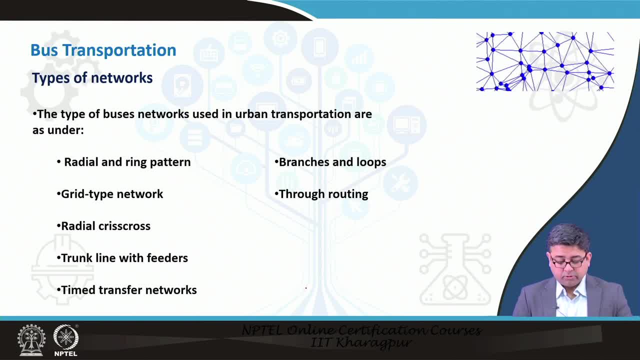 After you are aware of the types of buses, now you should be learning more about the different types of bus networks. So when you, when you visit a different or a new city in the next time, try to get hold of a public transportation bus network map, or maybe even look up on the internet to see. 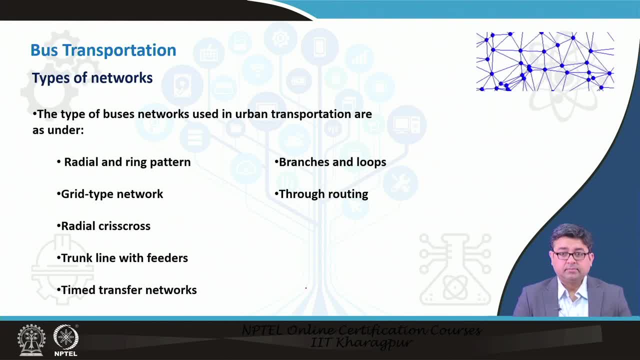 you how the bus network is or the transport network is public transportation network is. You would see that there are different types of patterns of these transportation systems or bus transportation systems. Listed here are few of them that are mostly used worldwide: Radial and ring patterns. grid type network. radial crisscross trunk line with feeders. 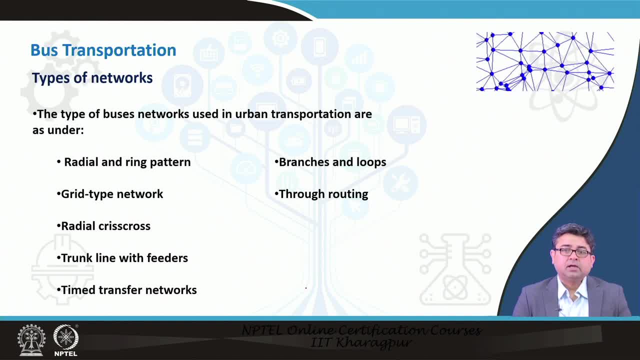 time transferred networks, branches and loops and through routing. So we there is enough Material in the textbooks available that will tell you about these routes. different types of route networks. The most common ones are the trunk and line, the trunk line with feeders, branches and 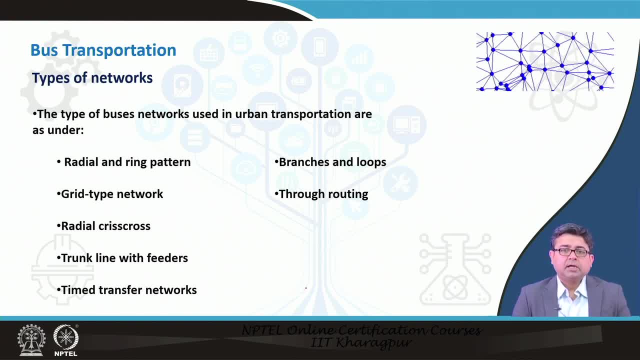 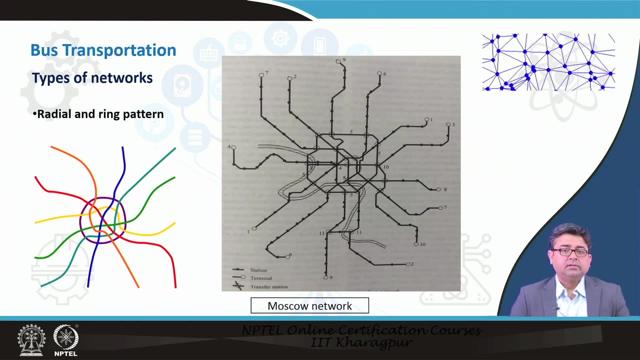 loops and the grid network. Radial and ring pattern is also fairly popular across different cities. So if we look at some of them in detail, So you will see the radial and ring Ring pattern somehow looks like this. So it has a radial pattern which radiates out of the central business district. ok, 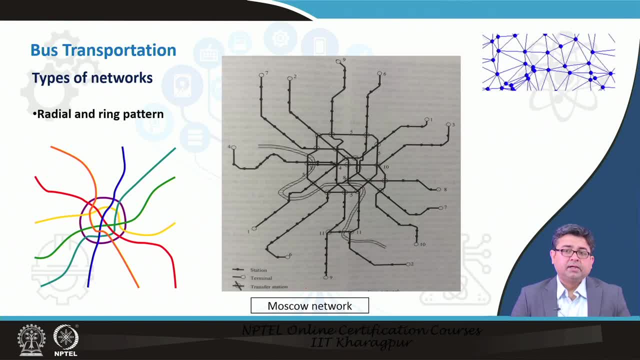 So all of the different routes radiate out of the central business district into the different suburban areas, but at the same time it is overlaid- overlaid by a radial network as well. So why is this usually done? Because now, if you want to travel from, 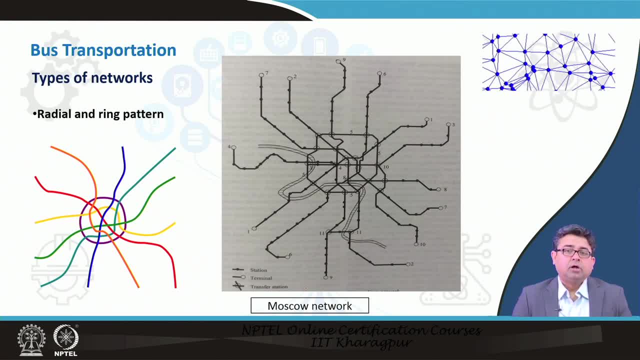 Ah, the central business district, on on the blue route and then. but your destination is eventually on the green route You do not want to be. There is usually no connection. if there is no radial, if the radial route is not there, there is no connection between the blue route and the green route, except for going all the 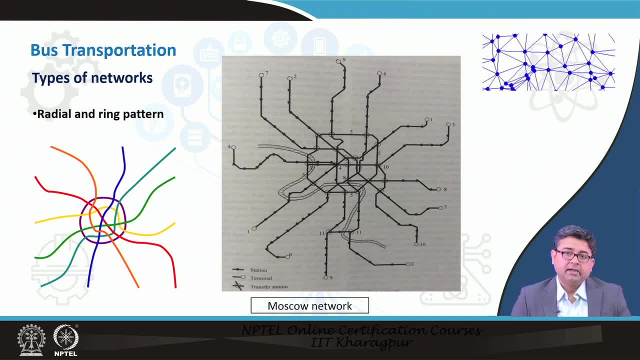 way into the C, V, D and then taking a green route again. So this radial pattern kind of allows you to now transfer between between these different types of routes or different types of lines. So that is the a pattern that is observed in many of these cities. An example here shown is the Moscow. 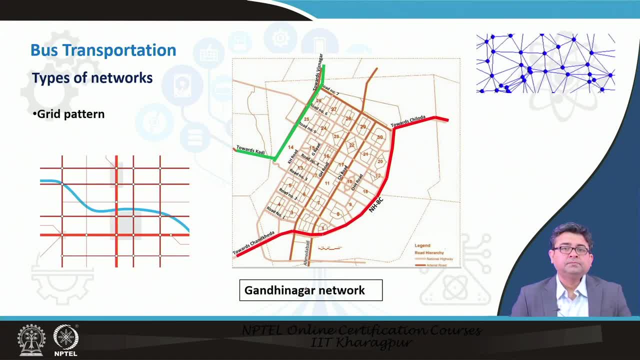 cities network. Grid network is something that many of you would also notice in some of the cities that have well planned road networks. Well planned road networks, as in ah, road networks that are square or rectangular in pattern. So if you have such grid patterns, it is very easy to ah, ah, reach your destinations. the 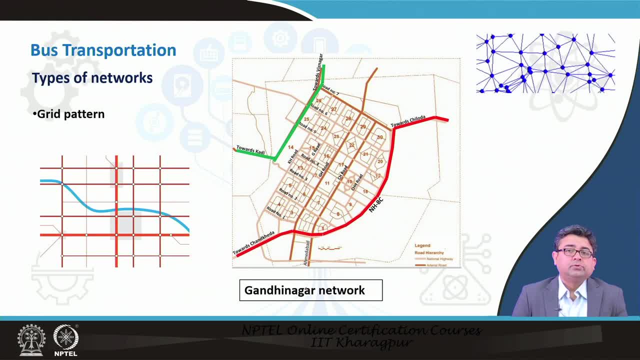 block sizes usually are very small. So once you get off of your bus, ah, your destination is not very far, or your origin is very close to your ah bus stop, ah, at the ah home end of it. So, ah, these are. These are mostly restricted around the CBD areas of most of the cities now. So, ah, the 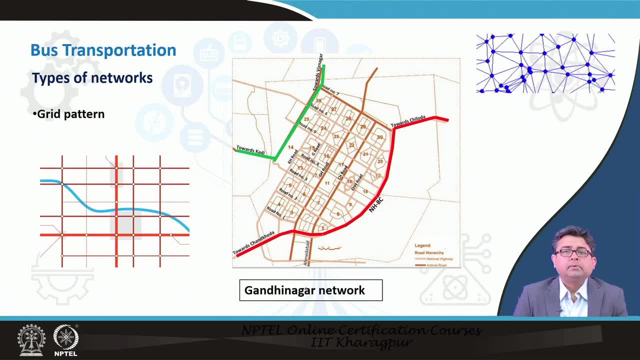 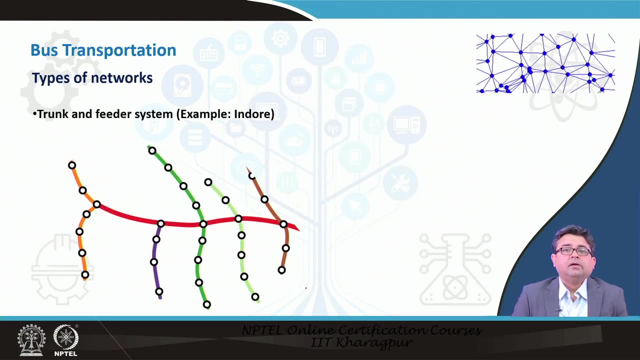 CBD areas tend to have ah kind of a grid ah road pattern and hence the bus routes in the CBD areas also tend to have a ah, very ah grid pattern of network. Shown here as an example is the Gandhinagar network Moving ahead. ah, this is something that ah is. 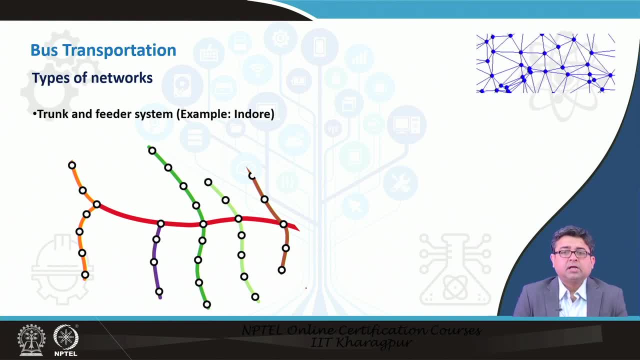 becoming ah is popular Worldwide also but is now catching up in India, especially when there are BRTS corridors, ah bus rapid transit system corridors. So an example is the Indore city ah bus rapid transit corridor. So the red line, that is the trunk line, ah is the trunk or the main. 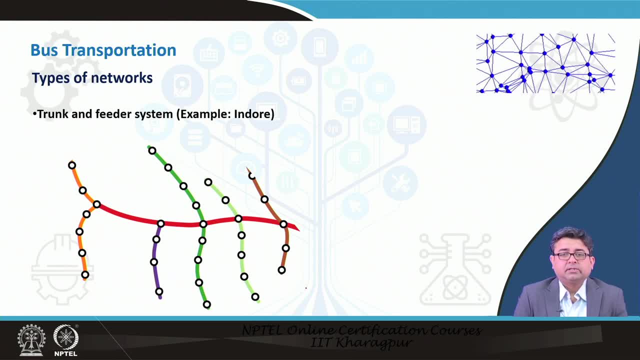 line that runs, ah, either east west- in this case it is shown east west- but can run north, south as well. So that is the main route that runs. and then there are different feeder routes to that main or trunk route that feed into this main line. So the here you would. 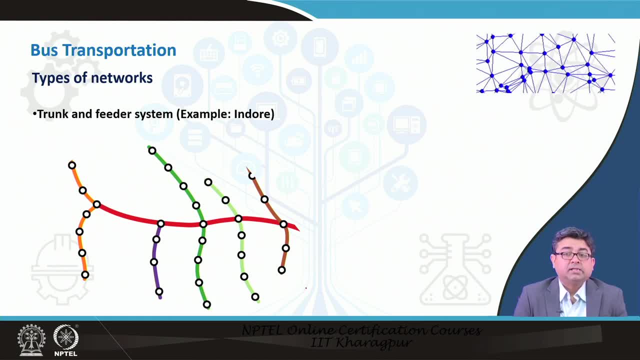 see that there are different green, orange, ah brown lines that are feeding to the trunk line. So this ah, this type of network usually is seen when there is a main BRTS system and then there are different ah feeder routes that feed into that system. 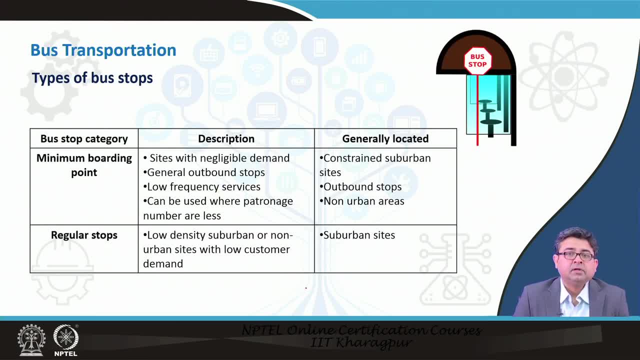 So what if the, if a particular stop ah has very heavy ah ah boarding during the morning times and very heavy ah ah deboarding during the evening times, then you would know that that is a very ah ah, maybe a major residential area where people in the morning are going. 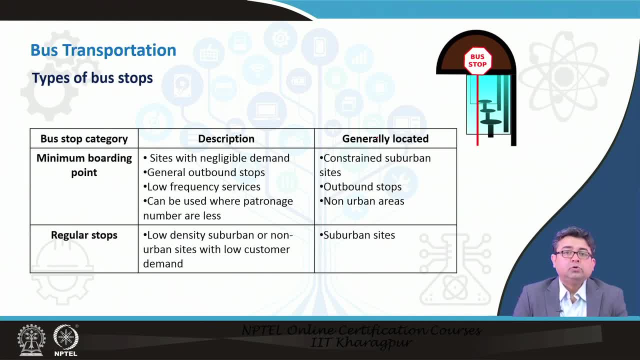 to work and the evening are coming back, So you would have them as regular stops or sometimes priority stops. even So, you would see that the bus stop category categories are divided into different categories and ah generally based on the location where they are. So the first one are called minimum boarding. 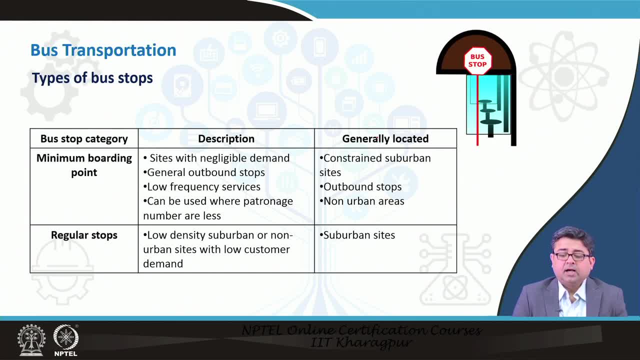 points which have very little demand ah. they are maybe ah suburban locations ah, which in the during the day time has very ah low demand but may have a little bit of demand during peak and off peak times. So those are minimum boarding points and why you want to ah classify. 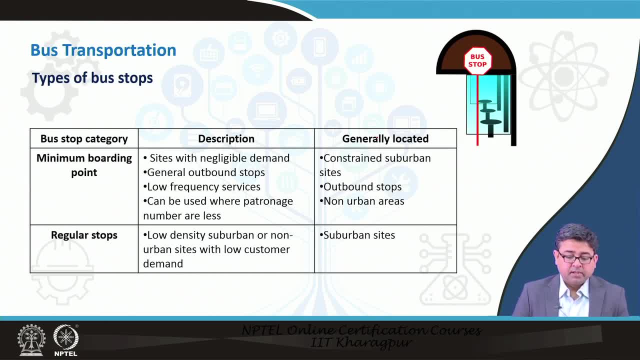 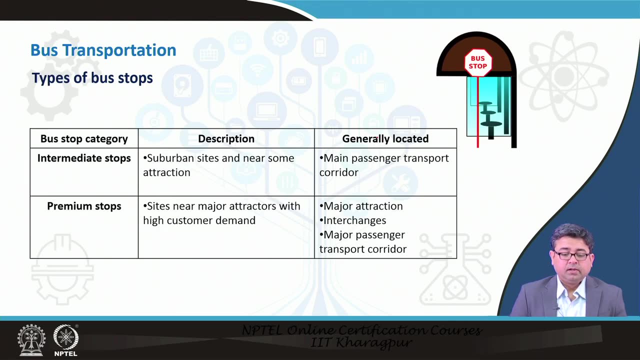 them. we will ah get to it a little bit ah later. Regular stops are ah regular suburban sites. that ah we discussed just now has morning, morning peak and evening peaks and usually very little demand in the mid ah in the mid day. Intermediate points are maybe ah suburban sites. 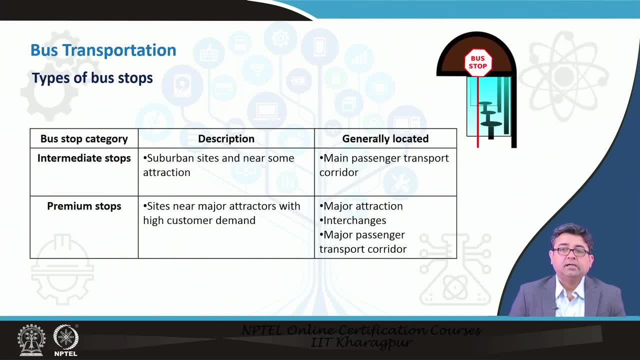 near some attractions. So maybe there is a park and ride lot or there is a some kind of a- ah, large, ah- Shopping center in the suburban area. those, those are classified as intermediate stops, whereas, finally, premium stops are the site, are the stops near major attractors, ah, big. 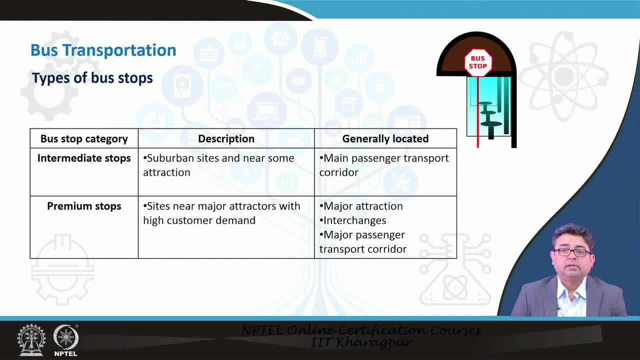 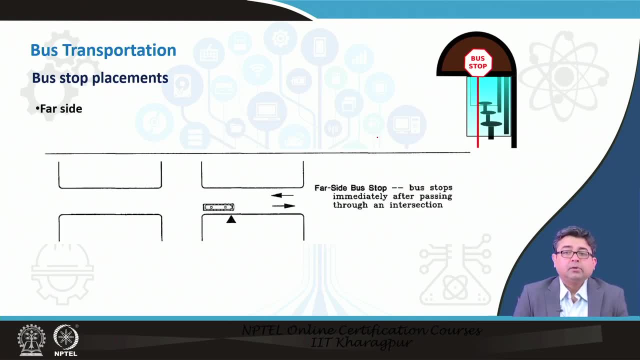 office complexes, ah big ah entertainment places, or so on and so forth. Now, after knowing, ah, what are the different categories of bus stops, one also has to know where to place these bus stops on the road network. That plays a very important role, because, ah, these are the ah locations along the ah road network where the bus is going to ah. 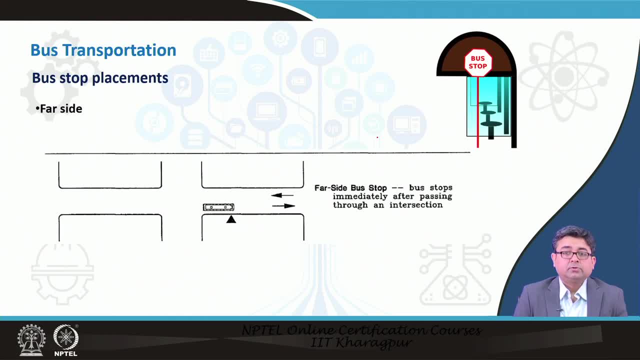 stop to pick up and drop off passengers. So the location has to be very ideal, otherwise it may not be able to serve the community. at the same time, the location should not ah cause much delay to the traffic. So that is the important role, because these are the locations along the road network. 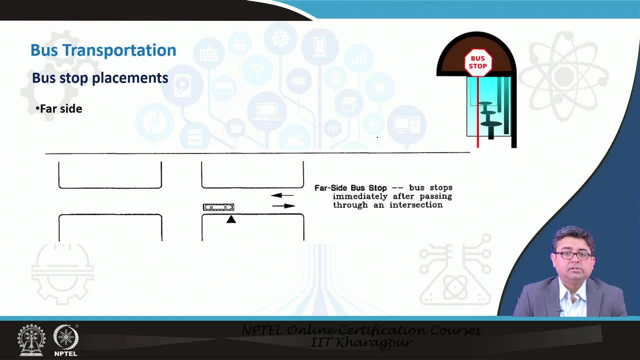 and the traffic to the other traffic modes that are applying on the street. So here is ah, an example of ah, where a bus stop can be placed. If you look at ah, this street network, this is an intersection and it is shown here that the bus is the bus stop. 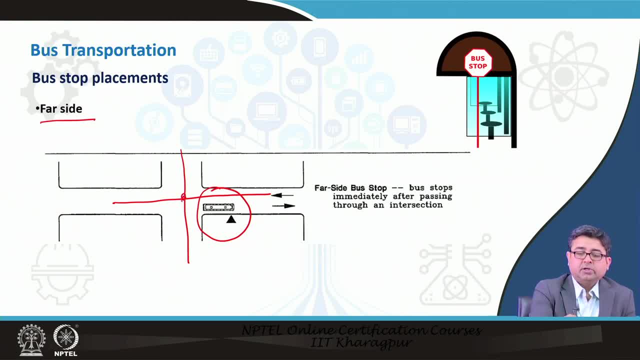 is on the far side of this intersection. So if that is the intersection and the bus stop is after the intersection, then it is called a far side bus stop immediately after passing through an intersection. So this is called a far side bus stop, Whereas a near side. 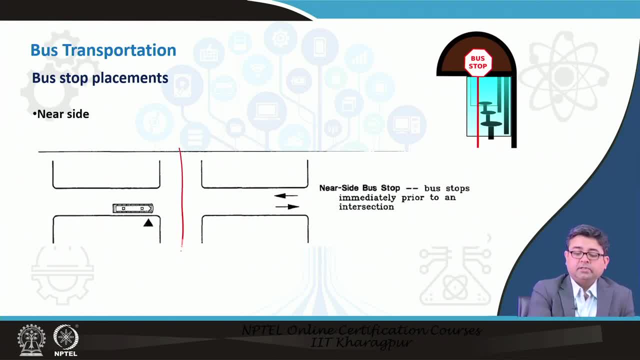 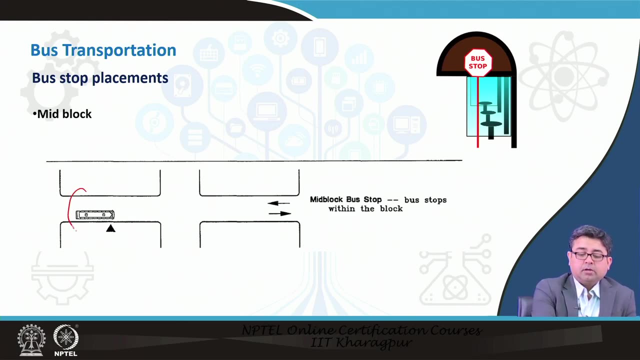 bus. a near side bus stop is just the opposite. So if this is the intersection and if the bus stop is before the intersection, Then it is called a near side bus stop. So this bus stop. And the third category is a mid block bus stop. So mid block bus stops is: 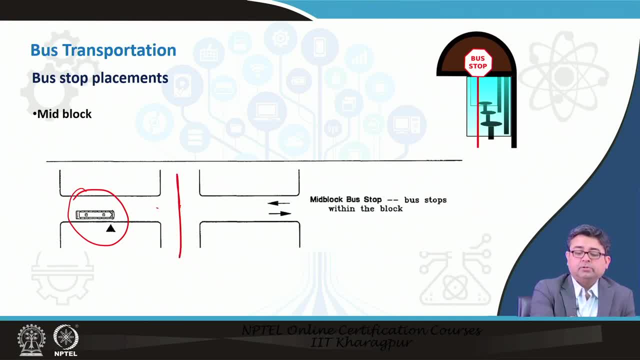 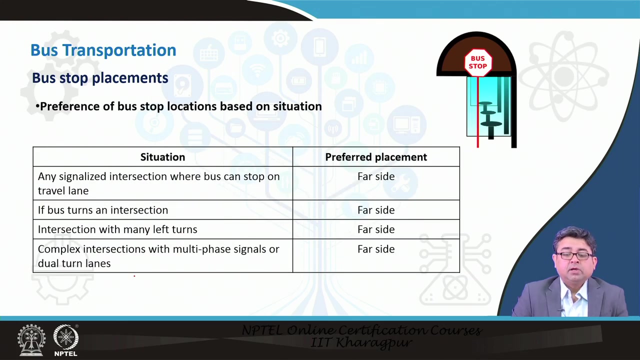 it is neither close to any of the two intersections. it is neither close to this intersection nor this intersection. it is somewhere in the middle of this block. Now that we have these three different types of bus stop locations, one also has to understand when to locate these bus stops at these three different locations. So usually you would: 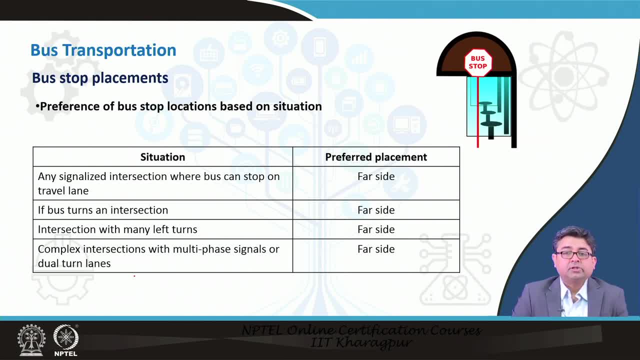 see that the preferred location of any bus stop is on the far side. So there are different situations when bus stops are preferred to be placed on the far side, such as any signalized intersection where bus can stop on the on the travel lane. So, as you would see here, 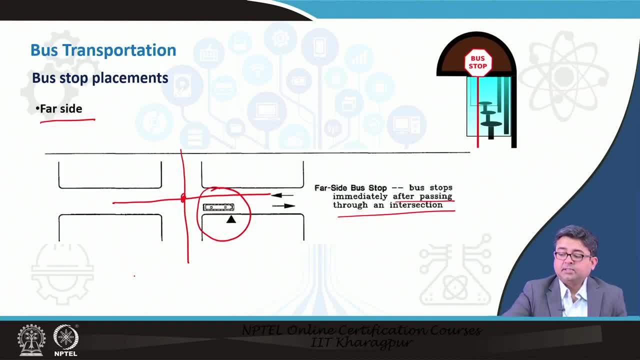 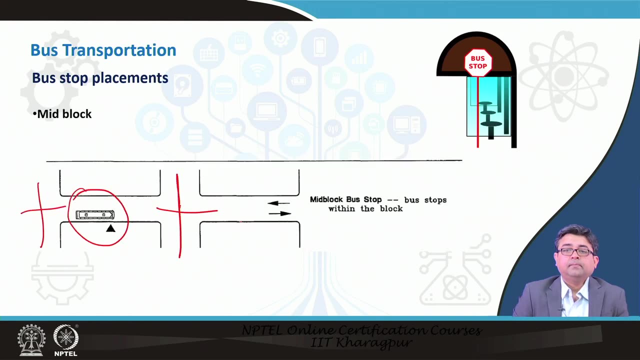 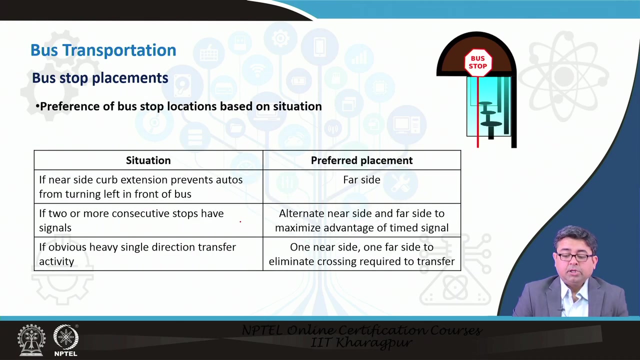 in the previous slides- bus. the bus is on the travel lane, stopping on the travel lane, So there are other traffic that is going on the same lane and the bus is also stopped on the same lane. Others other situations are given here you would very rarely when somebody would want. 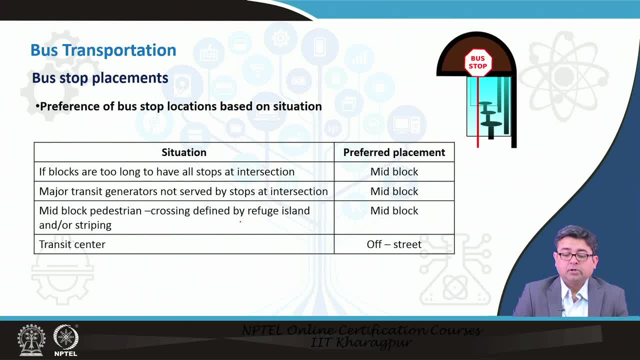 to place a bus stop. So the preferred bus stop in the mid block would be. if the blocks are too long, So if the distance between successive intersections is too long, then what you would really want to do, ideally want to do, is not have those bus stops at the intersection, but somewhere. 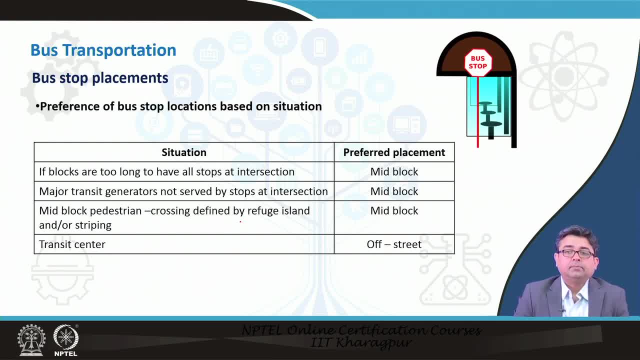 in the middle of the intersection, So that you are capturing all the possible riders that are in the middle of the block. Otherwise, it may be too long a distance for them to walk from their origin to this intersection. Also, the other last item listed here is the, a transit center which is off street meaning. 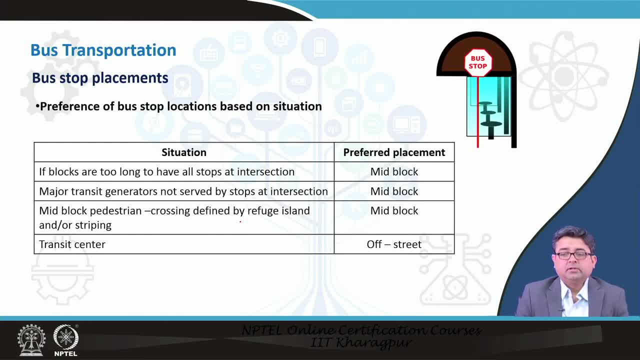 that it should not be on the travel lanes, it should have a different structure associated with it. So that is where the terminal stations of the transit centers, where there are multi modality transit centers involved, where you change from a bus to may be a train or some. 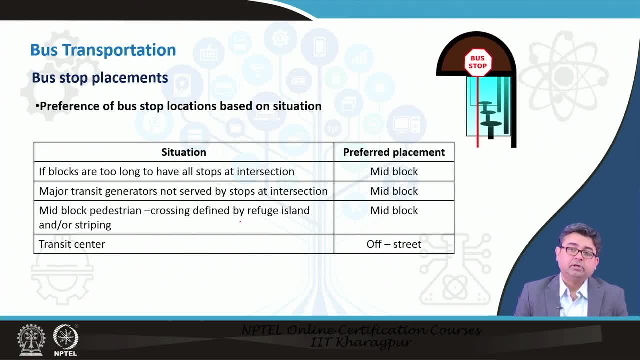 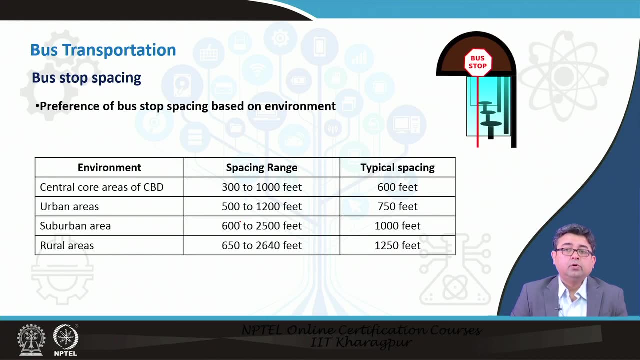 other for from a urban bus to a regional bus network. So those are called transit centers and those are usually have their own structures which are off the street. Now here is a typical bus stops pacing scenario. So now you know where the bus stops physically. 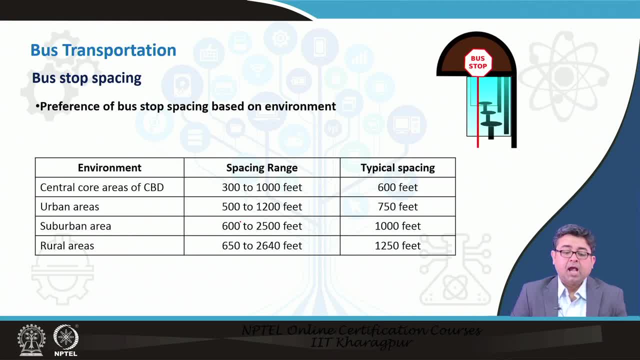 can be located either far side, near side or mid block. and now it is important also to know what is the spacing between two bus stops. So you would see that in the central code area or the CBD, the spacing is usually very less because there are lot of ah attraction. 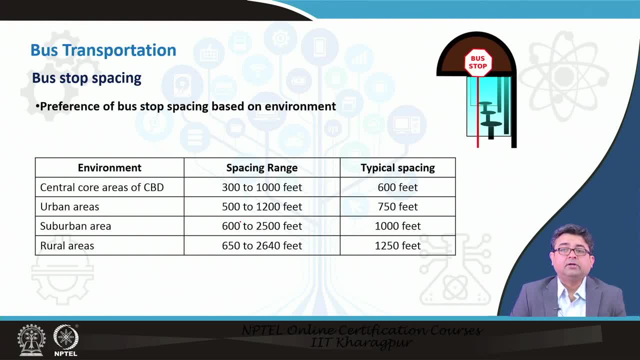 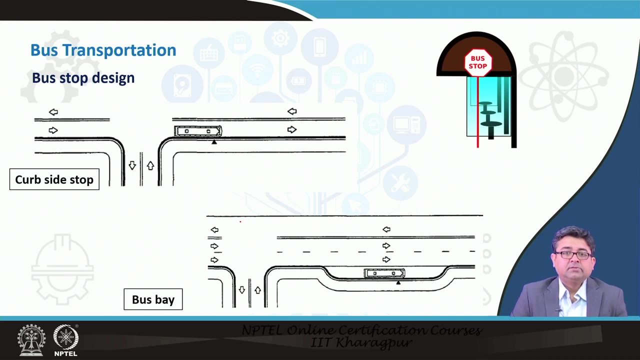 points and people may want to get up and get off at several locations. So your bus stops are usually spaced very close to each other when compared to suburban or rural areas, where you can have bus stops, Bus stops very farly spaced from each other, very distantly spaced from each other. Next, 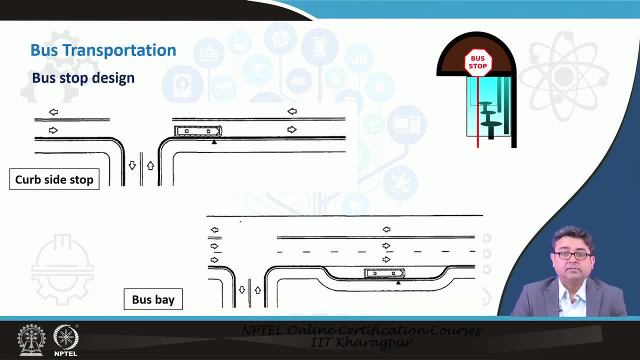 we come to the different types of bus stop designs. So now that you know where they can be located, it is also essential to understand how they have to be designed. So let us look at the most common type of bus stop design that we have also looked at- ah, while looking. 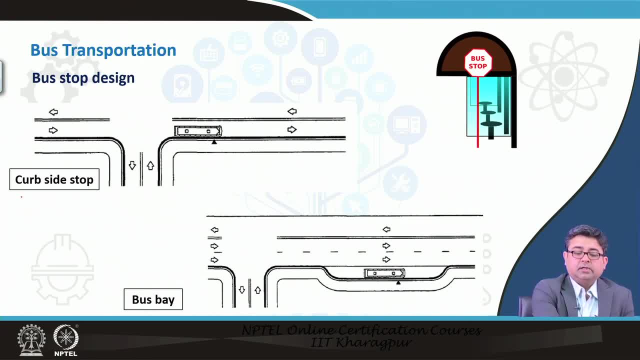 at the ah bus stop locations, which is the curbside stop. So a curbside stop this is a far side. if you remember, this is a far side bus stop which is after the intersection and it is also the curbside, meaning it is right next to the curb. 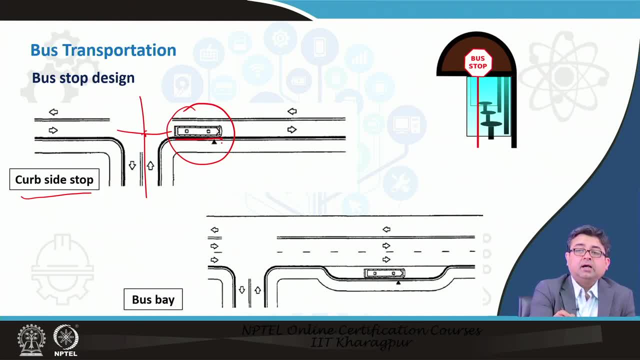 on the road, So it does not have any special ah infrastructure requirement. it just stops right next to the curve and people get on and get off from the bus, Whereas if you in certain other situations, you may have something called a bus bay. So here are your regular. 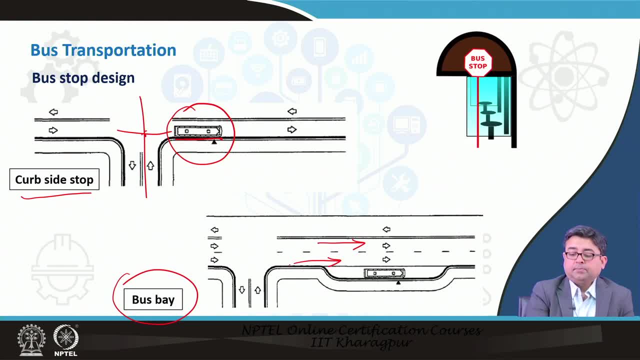 traffic lanes, but then the bus would get into this special lane which is called the bus bay, and the bus stop is located in this bus bay. So this is ideally ah done or required when there is a location that has a large number of boarding and alightings. So when 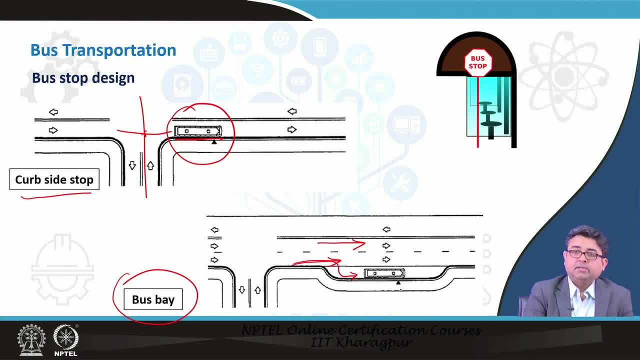 the bus has to really get on and get off from the curbside stop. So this is the curbside stop. So if you really stop for a or dwell time of the bus is very high, you do not want it to be obstructing other kind of traffic, which it would do if it was on a curbside. 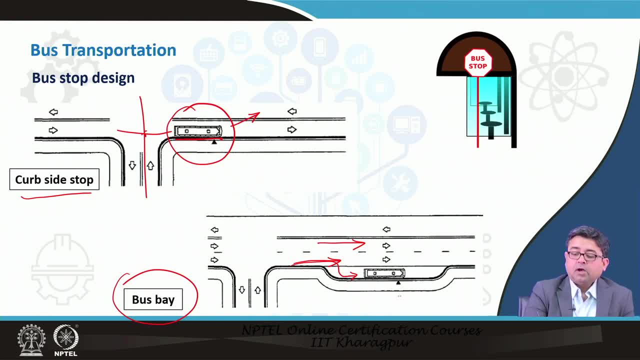 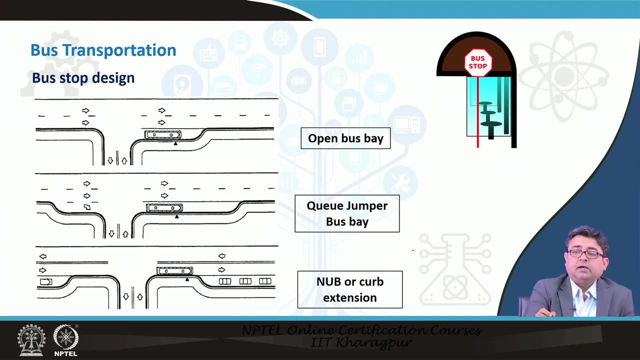 ah, if it was, if the stop was on a curbside. Now it has its own special bus bay, and so there is no obstruction to the ongoing traffic. The next one we usually call it is another, ah, variety of the bus bay lane. This is called an open bus bay. 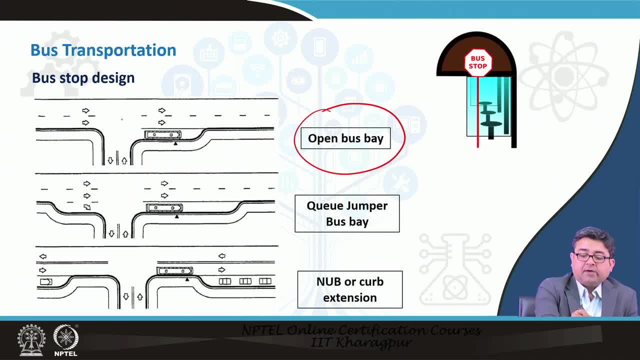 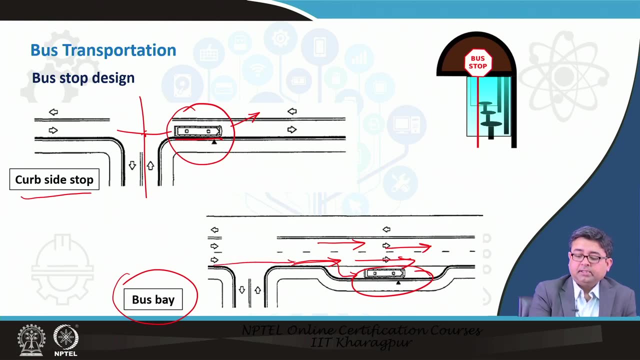 So you would see that actually right after the intersection the bus bay arrived. So the buses arriving directly gets into the open bus bay. if you look at at typical one here the buses go past the intersection in the travel lane and then the bus bay is a. 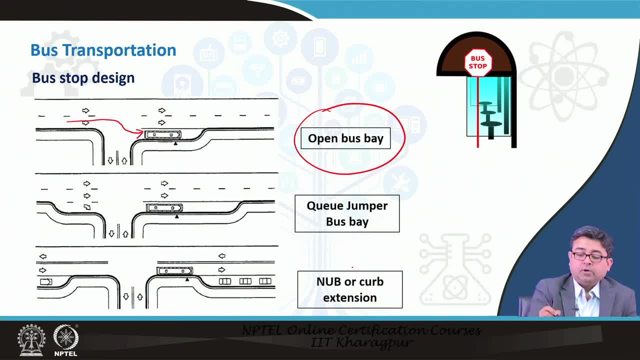 little bit later on, Whereas an open bus bay you the open bus bay, not very far outside of the traffic differences. So basically you would see a track coming in and then going, you, the bus can directly get in to the bus bay. There are different advantages and disadvantages. 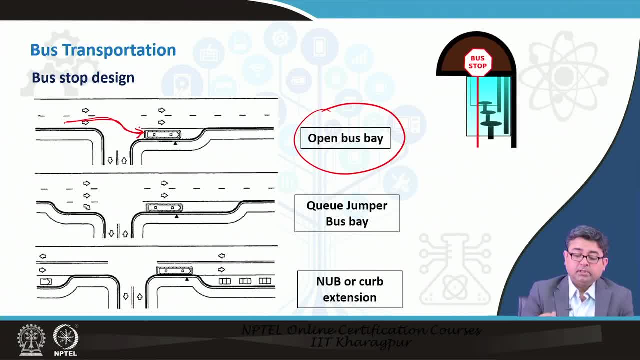 of this and when they should be designed is all available in the textbook. but first let us at least look into what are the different types. Then something designed that is called a queue jumper bus bay. So what happens here is if there is a dedicated right turn lane here. I mean, these are the diagrams are shown here. 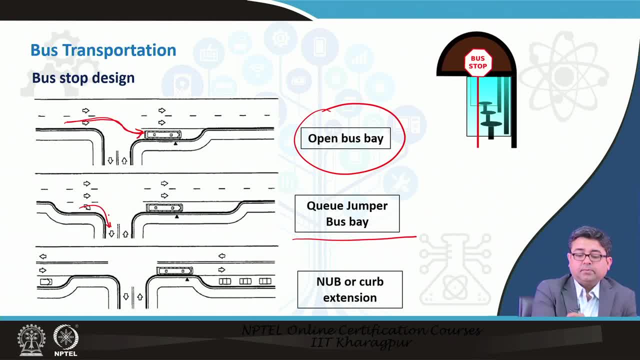 keeping in mind the western driving conditions, where people drive on the right hand side and they have free right turn lanes, So in our case it would be left turn lanes. So if there is a free right turn lane, what usually is allowed is the buses are allowed to take. 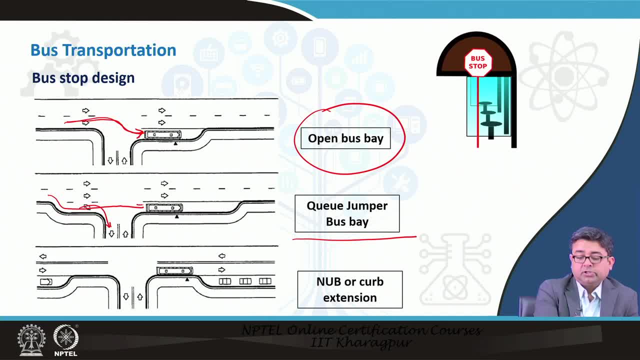 the right turn lane but jump the queue, jumper bus The queue and go straight. So otherwise they would be queued up here in the travel lanes and waiting for this queue to be dissipated before they could go ahead. So in order to 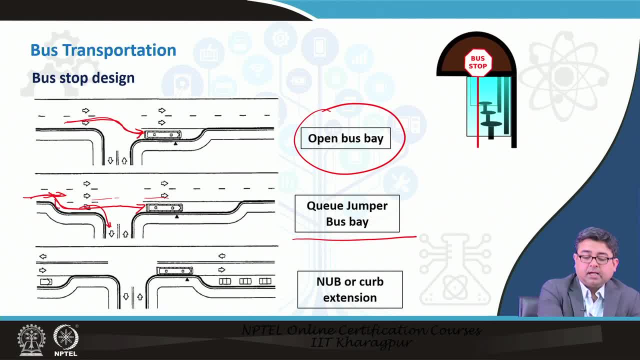 avoid them to be queued up on the travel lanes, they are allowed to take this right turn only lane, but jump the queue and come directly into the open bus bay. So that is the example of a queue jumper bus bay. Similarly, the last one is a. 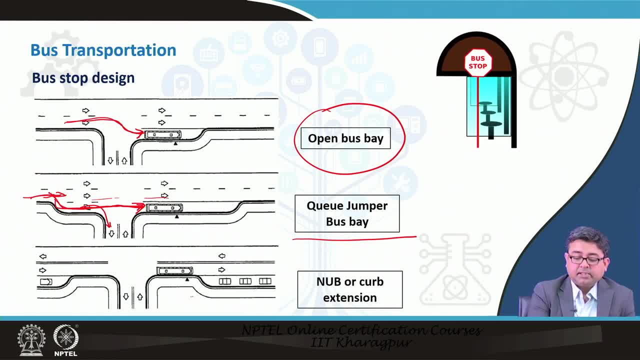 nub or a curb extension. What happens here is usually: the curb is supposed to be here. However, it is kind of extended So that the parked vehicles can be on on this side, the parking can be on this side and the bus stop can be here. So these are, ah, pretty. 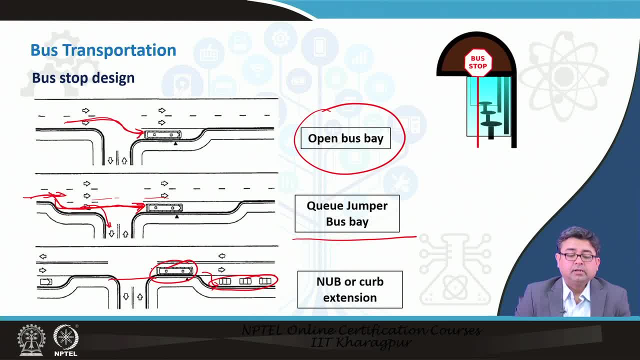 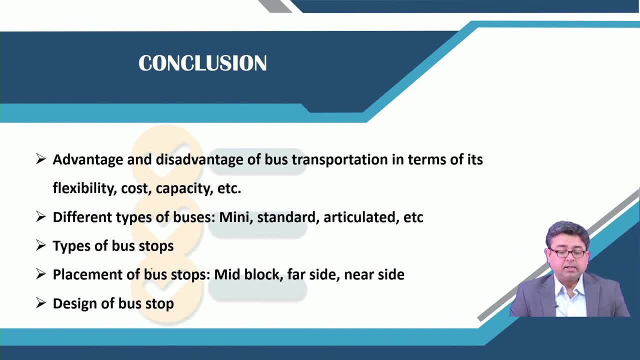 well illustrated and easy to understand and explained in your textbook. So, ah in conclusion, what we looked at ah today was: ah all the advantages and disadvantages of ah- bus transportation in terms of flexibility, cost and capacity. We introduced you to the different types of buses, different types of bus stops, the placement of bus stops as. 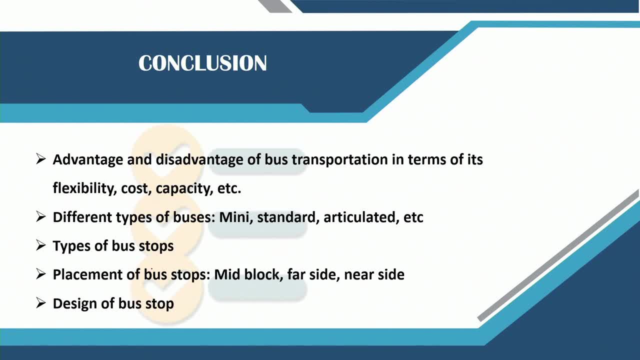 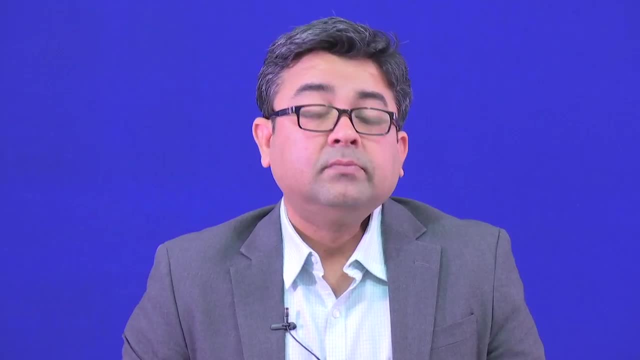 well as the design of bus stops. So all of these four or five elements together is going to help you to plan for a bus network in your city and make it more efficient. Thank you so much for your time. Looking forward to having you in the next lecture. . .